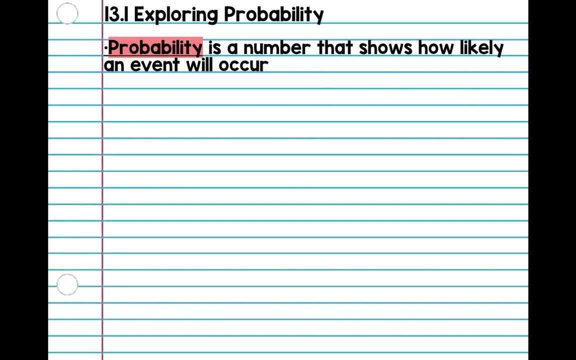 with our vocab. So probability is just a number. it could be a decimal, fraction or percent that shows how likely an event will occur. So in my case I said a 5% chance. so my number was a percentage and my 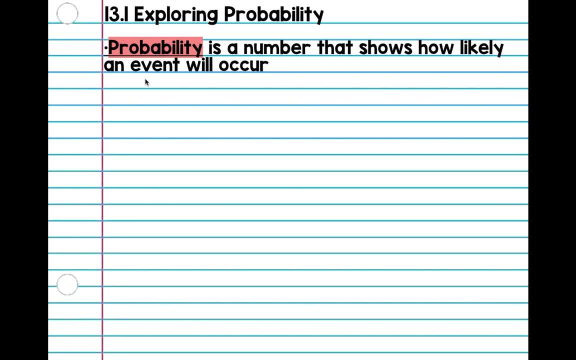 event was it snowing? So that's what the event is. The event can also be flipping for heads. that's the event, okay, So we're going to start with the first scenario. We're going to be using candy M&M's. 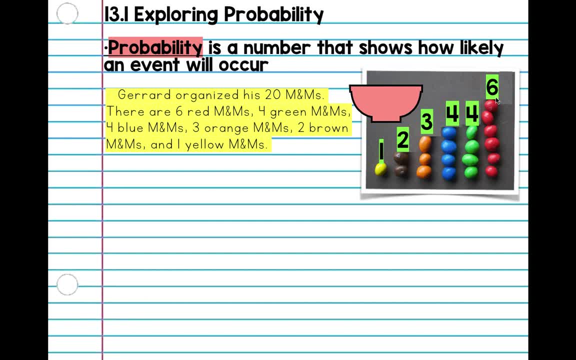 So Gerard organized his M&M's. He has 20.. There's six red, four blues and greens. We have orange, brown and yellow. So they're going to be asking you today and tomorrow to record the probability as a percent, just like what you did. 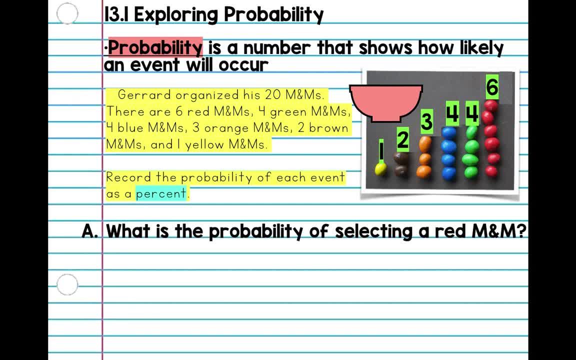 last week. But we're going to be working with easy numbers, So let's look at letter A. It says: what is the probability of selecting a red M&M? Okay, so we're going to look at red. We have red over here. So in grade six we're. 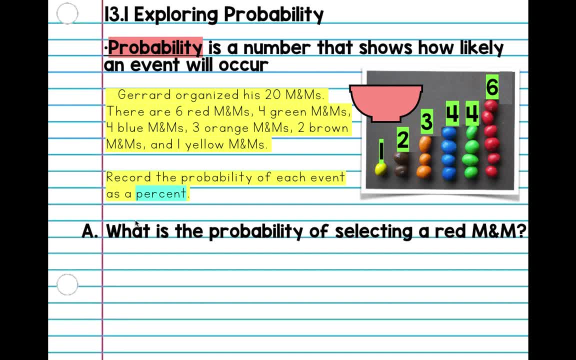 going to be using the proper formatting and I want you to copy this down. It looks confusing, but it's actually super simple. So this is how the formula looks: P parentheses. event: favorable: number of favorable outcomes, meaning how many there are over your total possible. 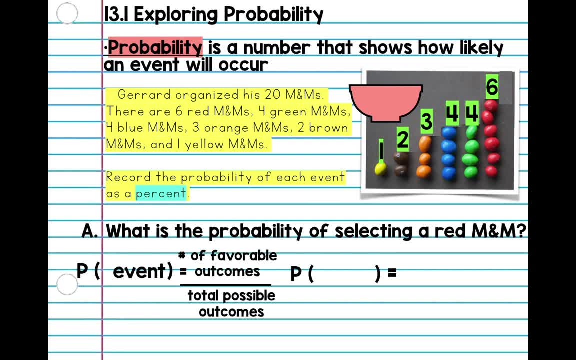 outcomes Okay, so let's put that in the question. So P, my event is a red M&M, So I put red And then number of favorable, meaning how many there are. So I just count: There's six And then my total. I know there's 20.. So six over 20, and there is my. 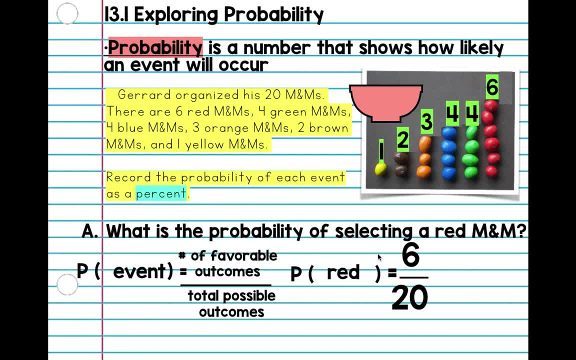 answer, But it's not finished yet. It's asking for percent. Okay, so if it asks for a fraction, then you can just put this, But it's asking for percent. So, like we did last week, we're going to go equals blank over 100.. And, just like what you know, 20 times 5 is 100.. So 6 times 5 is 30.. So the 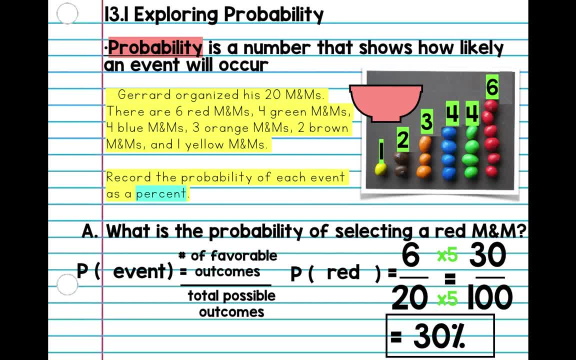 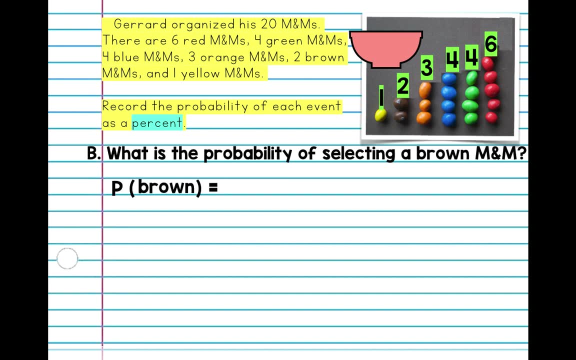 probability of selecting a red is a 30% chance. If I put these all in here, I have a 30% chance of getting red. Okay, All right, so let's try one more together. So I'm internet Width. I have Aaron Smith, So blue is the probability of selecting a brown M&M. So, P parenthesis, brown equals that one's easy 2 over 20.. And then 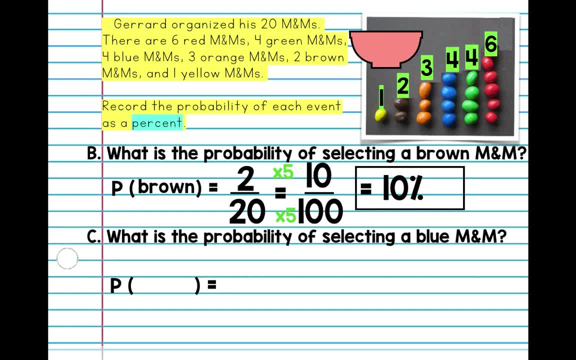 equals blank over 100, so I know it's times 5, so 2 times 5 is 10.. Oh, that's really small. So I have a 10% chance of getting brown. Not very likely, Okay. so P parentheses- blue equals 4 over 20, so multiply both sides by 5, you have. 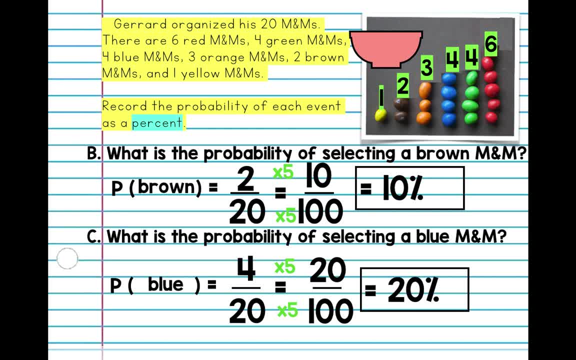 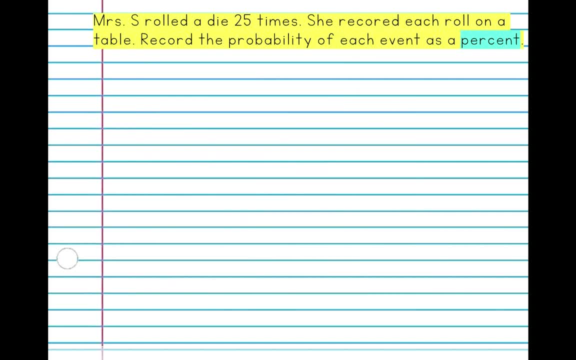 a 20% chance of getting a blue M&M. Alright, put a check mark if you got that- really easy stuff. So we're done with today's lesson. tomorrow's lesson is pretty similar. instead of having 20 candies, I'm going to have a dice, okay. 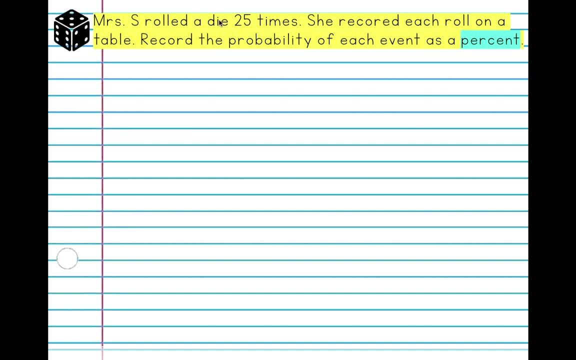 Oh, I'm sorry. a die, my bad. A die means it's a singular form of dice, so if you have 2, we call it dice, if you have 1, we call it die. Alright, so I rolled the die 25 times and I recorded it all on the table. 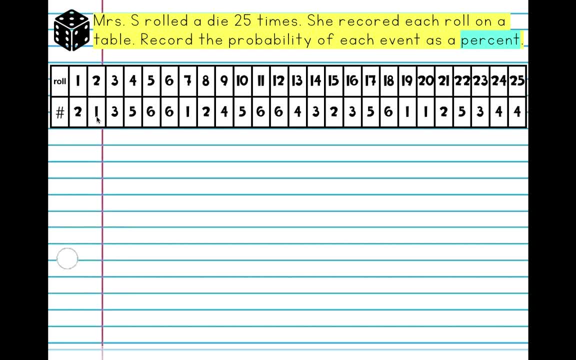 So if you look here, my first roll, I got 2,. my second roll landed on 1,. my third roll landed on 3, 4 landed on 5, okay, And etc. So now my denominator is going to be 25 and not 20, okay. 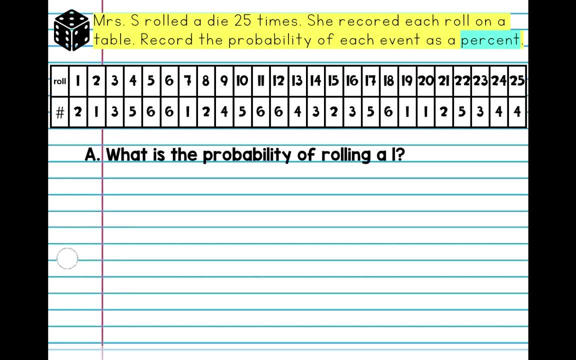 So it says: what is the probability of rolling a 1?? So you're going to go. So here you just have to plug in what we know. so P1 equals, and then we're going to count how many 1s there are. okay. 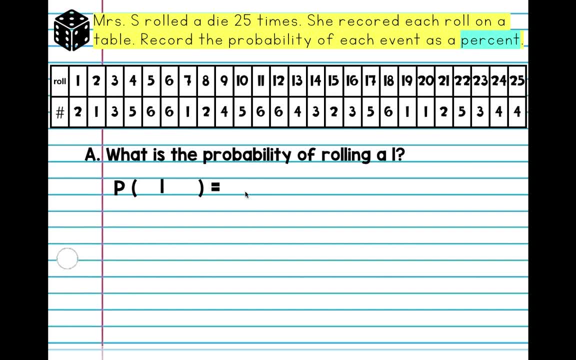 So 1,, 2,, 3,, 4.. So again your denominator is going to be 25, so we counted 1, 2,, 3, 4, so we have 4 over 25 equals blank over 100, and just like money, how many quarters are in a dollar? 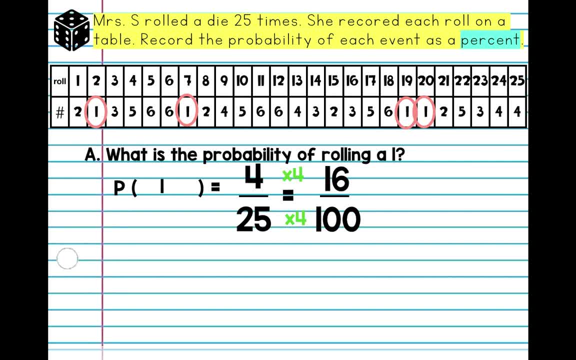 We know there's 4, so 25 times 4, do the same thing on top, I have a 16% chance of getting 1.. All right, pretty simple, right. So let's do the last question. go ahead and pause the video and do this one by yourself.